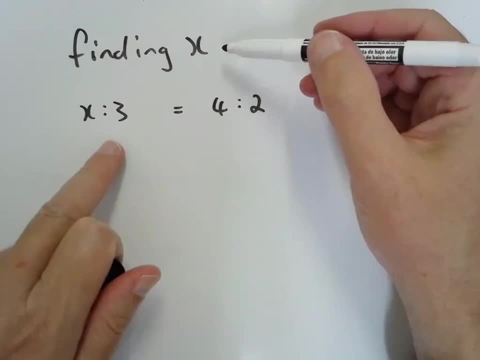 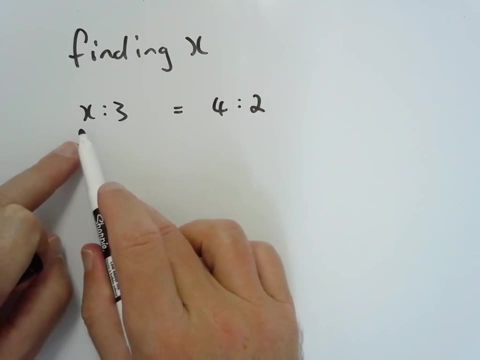 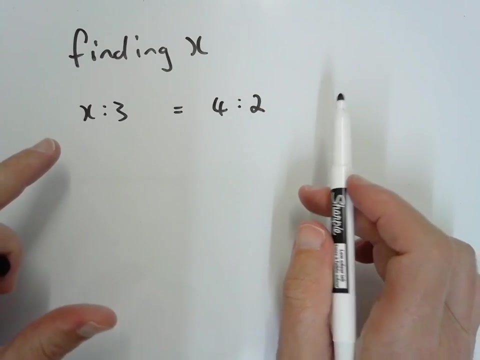 Okay. the second type of ratio is called finding x. So what we have is a set ratio- 4 is to 2, and we're looking for what does x need to be so that that ratio is the same as 4 is to 2.. Now you're going to say that x has to be 6,, isn't it? Because 4 is double 2,. 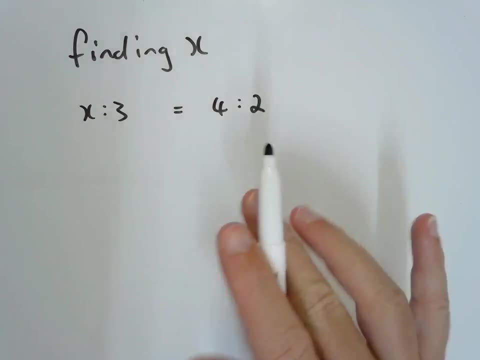 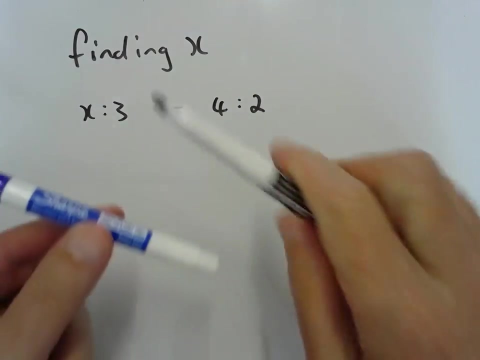 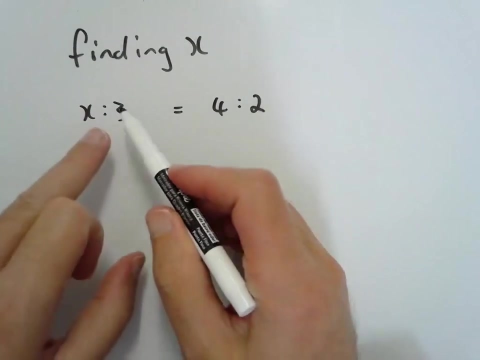 so it's double 3.. We know x is 6, but that doesn't matter. We need to know the process to find it. We're going to be thinking about the windscreen wipers in a car. When we turn them on, they go like that. So we're going to turn this into an algebraic equation using 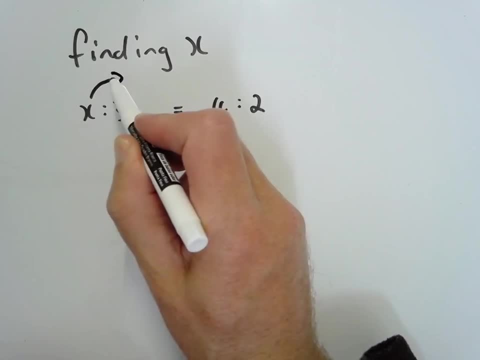 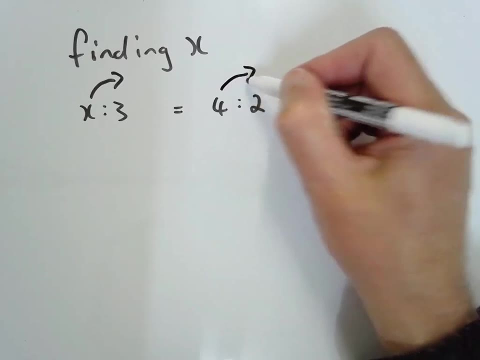 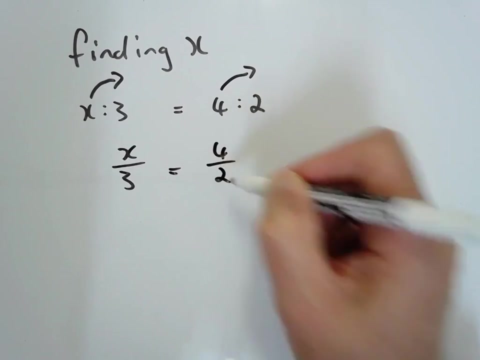 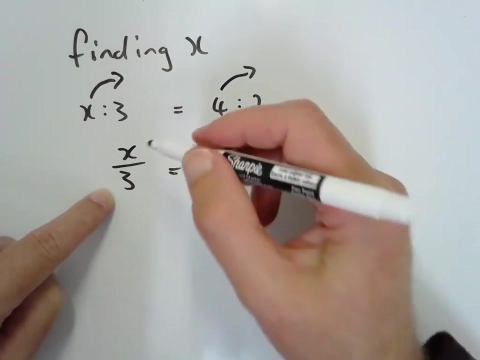 a windscreen wiper method. We want the x to go to the top. so if that goes that way, we want the 4 to go that way as well. So we're going to convert this To an algebraic equation. use algebra to solve for x To get the 3 to the other side. we 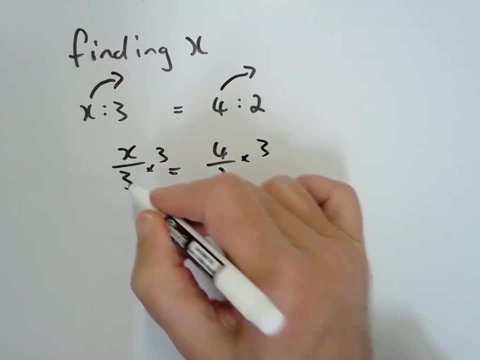 want to multiply by 3. That gets rid of the 3.. 4- 3's are 12, 12 divided by 2 is 6.. We're not surprised at that answer, but we're using a valid mathematical technique to get the. 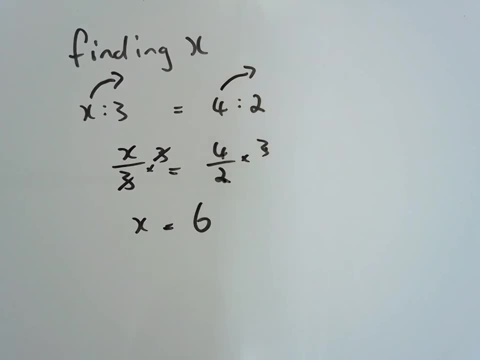 answer, not just whacking our answer in the test. Let's do another one, because these are pretty easy. Let's go, Let's put a word question in there. So let's just say: I've got a bottle of cordial and it says for every 5 litres. 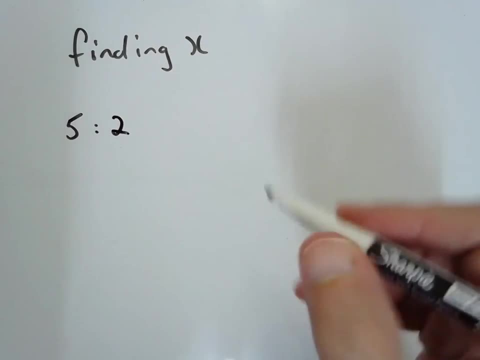 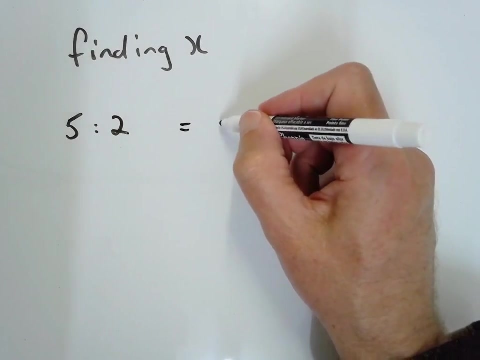 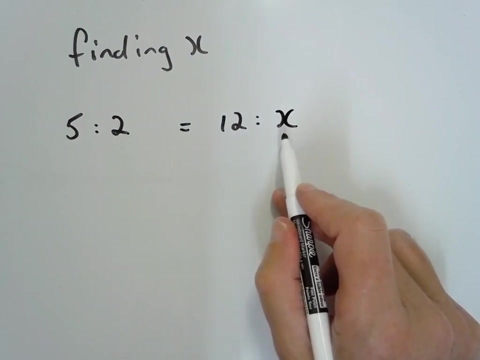 of water, you add 2 litres of cordial. Now I'm at sports day and I know everybody's going to be thirsty. I have got 12 litres of water and I want to work out how many litres of cordial. So water cordial, water cordial, and I want those ratios to be equal. 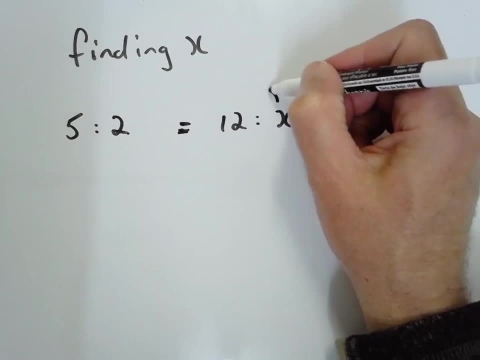 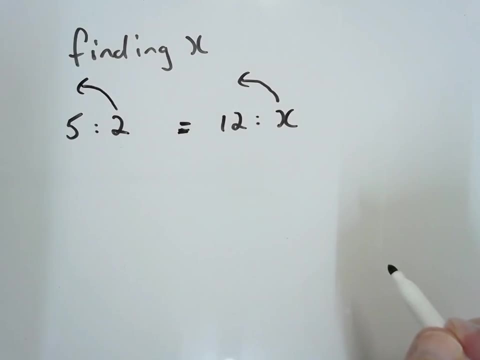 So windscreen wiper method, I want my x to the top. If my x goes to the top that way, and my 2's got to go to the top that way. so my equation's going to become 2 on 5 equals.